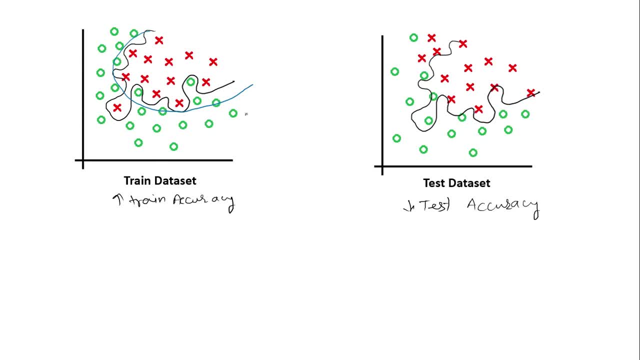 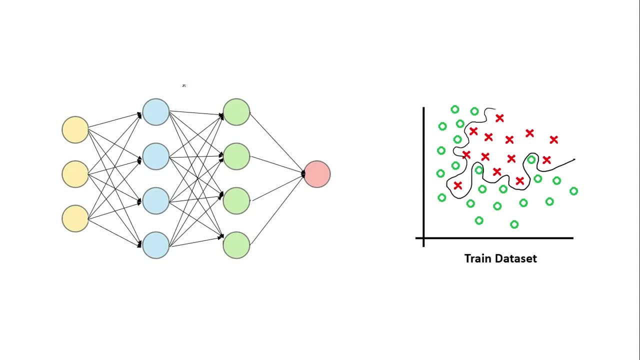 test data set. So to do this, we use regularization. Let's say, if you are using a neural network, then this highly complex non-linearity could be the result of having a very deep neural network which has many, many hidden layers, and each hidden layer. 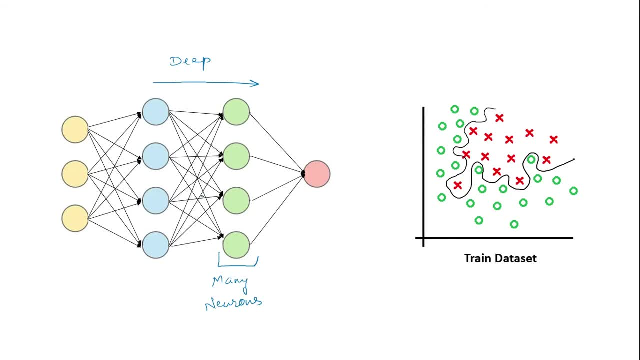 has many neurons. So all the complex connections between each neuron will create a highly complex non-linear curve like this. So if we want to somehow increase the linearity or to have a smoother curve here, then we would want to have a slightly lesser number of neurons. So let's say: 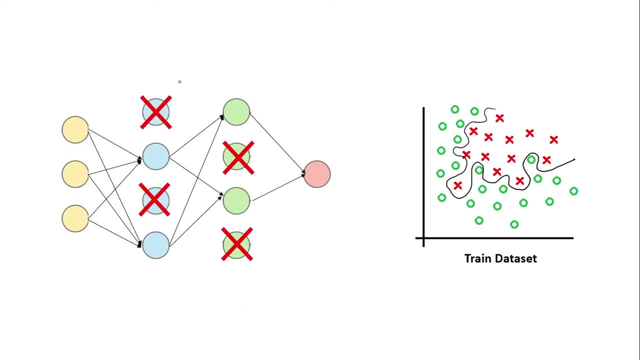 somehow, if we can get rid of certain neurons in the neural network, or better say, nullify the effect of certain neurons in the HG Pizza machine, that could consider this natural nourishment in the还是. you can have a slightly smaller number of neurons compared to the aprender jaki tumor. 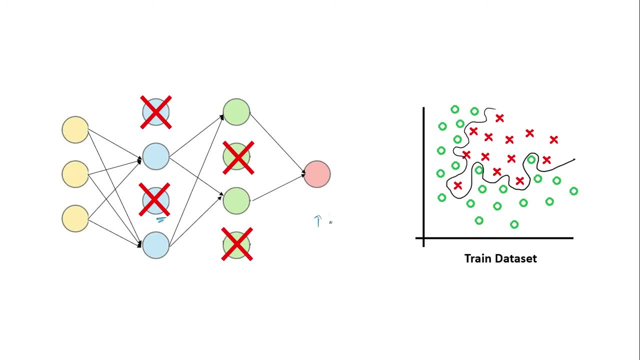 So let's say somehow, if we can get rid of certain neurons in the neural network, or better say hidden layers, then we can increase the linearity and thus have a better, smoother curve that will fit properly. A better way to understand is by taking an example of a regression problem. 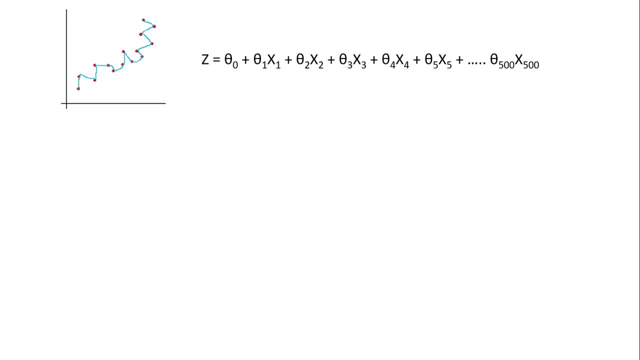 Let us assume that, instead of a neural network, we are making a regression model, and overfitting in this dataset will be something like this complicated curve where our model will try to fit on every data point of this dataset. This complex curve is only possible if we have so many number of parameters and, comparatively, 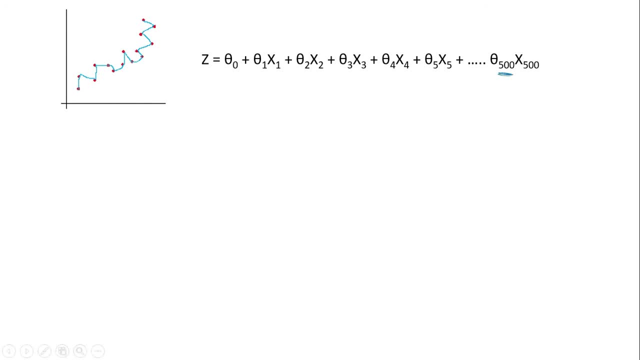 less dataset. So let's say, here we have 500 parameters, and if we had only one feature and or, let's say, two parameters, then it is only possible to fit a straight line in it. So this is highly linear. What we want is a middle ground between these two curves, so that we can have a 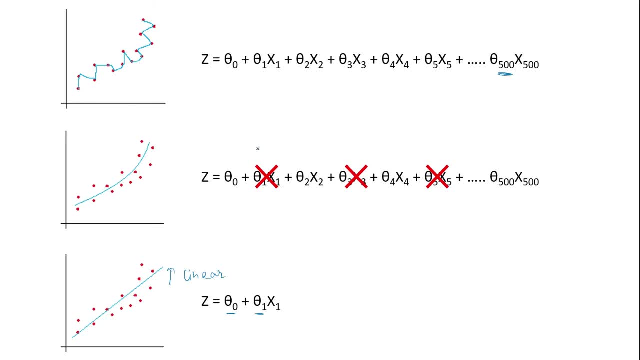 problem. We want a proper curve that fit well, and this is possible by eliminating, or better say, nullifying the effect of certain parameters or certain terms in this curve, so that we can have a better, smoother curve that fits like this properly. and this technique to nullify.